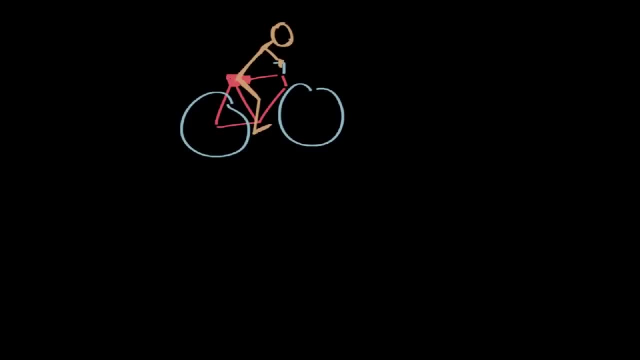 So sometimes I go for a pretty long bike ride and when I do that I usually end up kind of getting an ache in my lower back or in my neck, kind of from being humped over the handlebars for a really extended period of time. and when I do that if it's really bothering me, sometimes I take 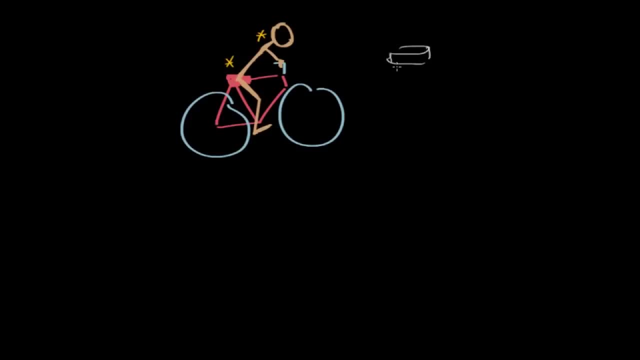 some medication for it. So some medication, and the medication that I prefer to take would be an NSAID. So an NSAID- and you might have heard of some common NSAIDs- You might even take them too. Aspirin, for example, is an NSAID. Aspirin and ibuprofen is another. 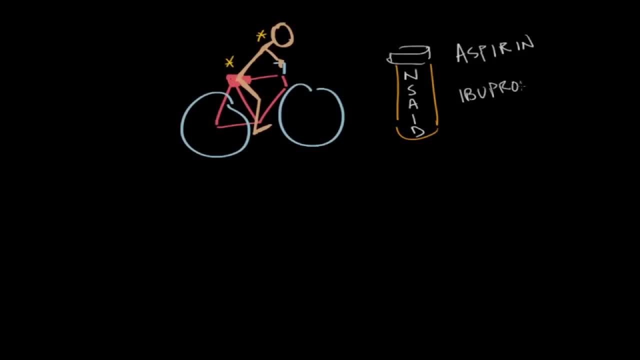 example, Sometimes that's called Motrin, but it's the same thing- Ibuprofen. But these drugs they help reduce that ache, because that ache is caused by inflammation in the muscles of my lower back And in my neck And these are anti-inflammatory drugs. In fact, NSAID stands for non-steroidal. 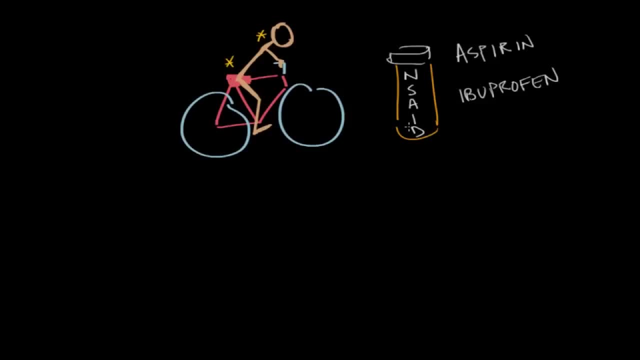 anti-inflammatory drugs, And part of the reason why these medications stop that ache is because they stop the production of prostaglandins. So prostaglandins, You see, prostaglandins are leping molecules that help signal inflammation. So if I can stop these prostaglandins, then I can stop any sort of inflammation that's in my throat- regular inflammation or navel inflammation. You see, prostaglandins are lipid molecules that help signal inflammation. So if I can stop these prostaglandins then I can stop any sort of inflammation that's in my neck. When you're. 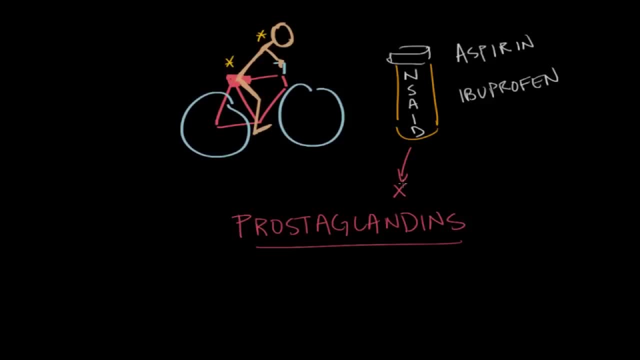 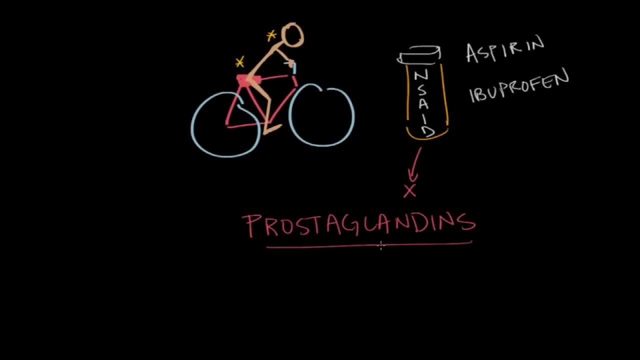 ользing anti-inflammatory drugs, you have to use mannset Vou Paulo, the SI grain, so that you can the kind of further and to some extent the past production of this inflammation and its effect on my body, which would be the ache Prostaglandins fit into a larger 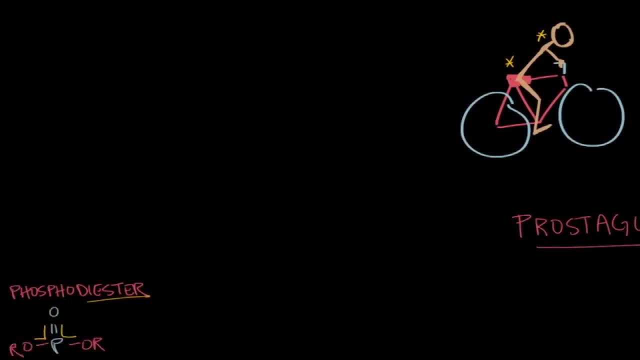 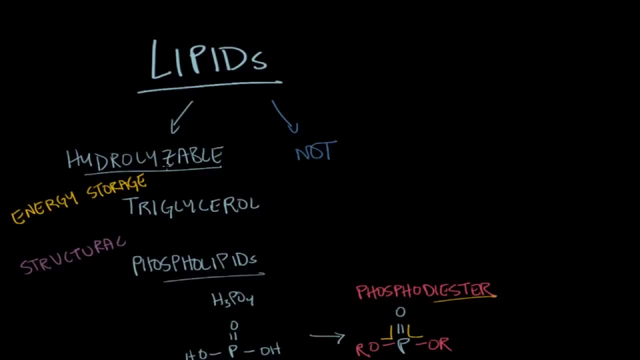 class of lipids called non-hydrolyzable lipids. Remember that we broke lipids down into hydrolyzable and not hydrolyzable. Hydrolyzable are the lipids that can be further broken down into smaller units through. 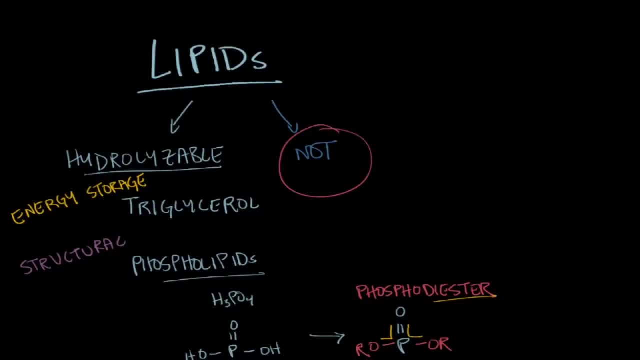 hydrolysis reactions, and then we have the ones that can't be. Prostaglandins fit into this kind of category of non-hydrolyzable lipids. We talked about how the hydrolyzable functions might include energy storage and this structural function, while the 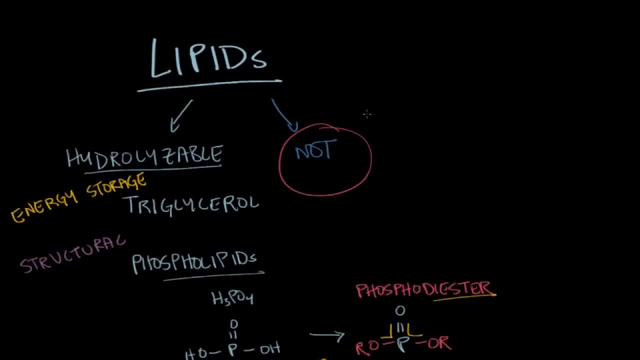 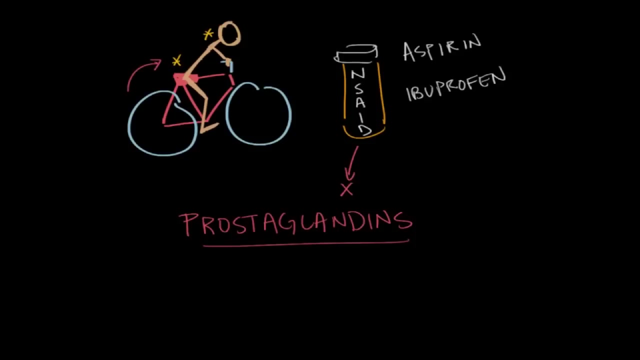 non-hydrolyzable lipids. their main function revolves, at least in our body, around signaling Signals, just like the prostaglandins signal this inflammation. up here I think I have a picture of prostaglandins that I can kind of fade in for us. 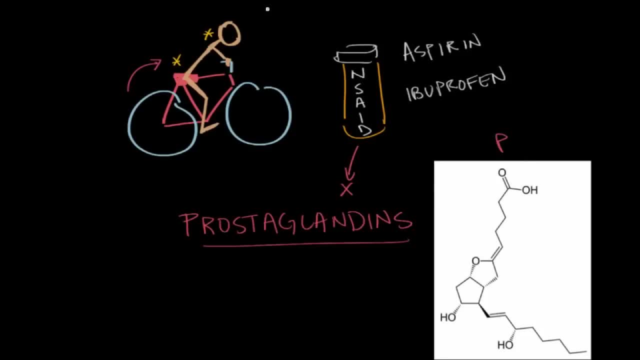 This would be the prostaglandin PGI2 here. Prostaglandins are probably the most notable of a group of biologically active compounds called eicosanoids. Let me kind of write that in here. Eicosanoids- Posi- is actually Greek for 20, so these are compounds. 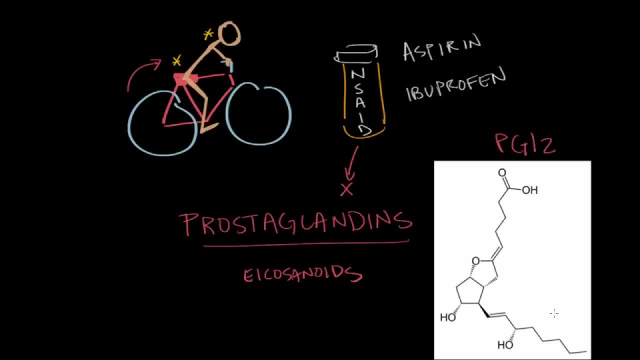 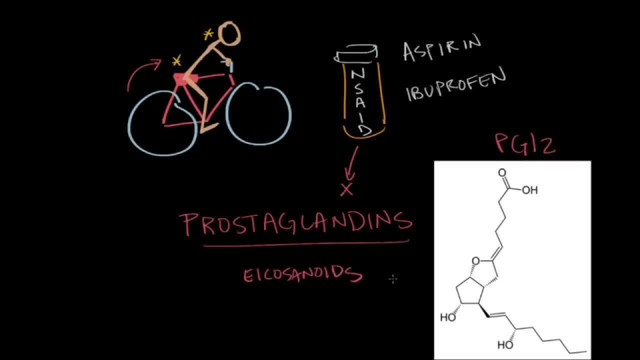 They also lower your blood pressure. prostaglandins, let's see, they lower your gastric secretions, they inhibit platelet aggregation, but there are a lot of signals, or effects at least, that are signaled by these prostaglandins. So they're a signaling lipid. 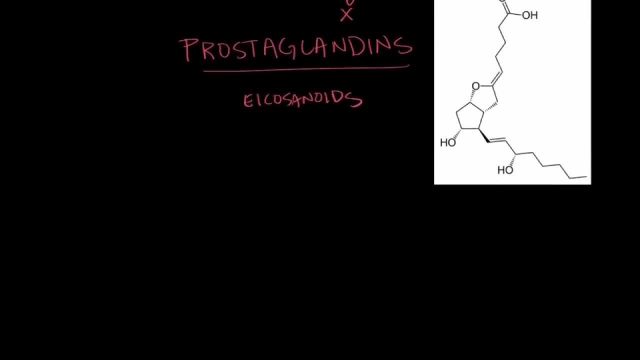 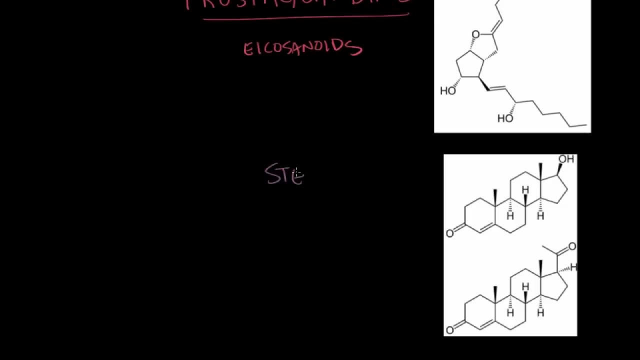 Now another signaling lipid that are kind of pretty famous- let me pull in a picture of them- are steroids, So I'll write that in as well: steroids. So steroids are tetracycline lipid, which means they have kind of four rings, four cyclic. 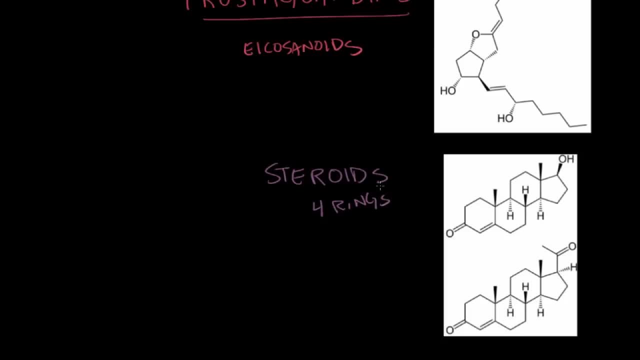 rings, and you can see this in the picture here. maybe I'll get a darker color. So we'd have one, two, three and then four rings and in each of these steroids the four rings. three of them are six-membered rings and the fourth is this kind of five-membered. 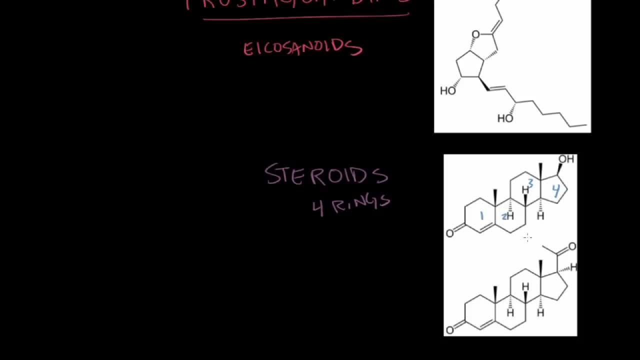 ring here. They all have this four-ring structure and then they differ in their little substituents. but I've already done kind of an in-depth series of videos on the structure and functions of steroids. but I'll keep it brief here and just kind of mention that steroids are another. 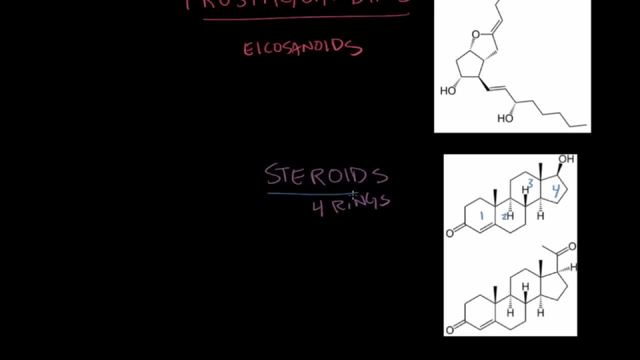 non-hydrolyzable lipid that have a signaling effect on our body. so cholesterol would be a steroid. So this one right here is actually testosterone and this one is progesterone, and these are examples of sex hormones in our body. 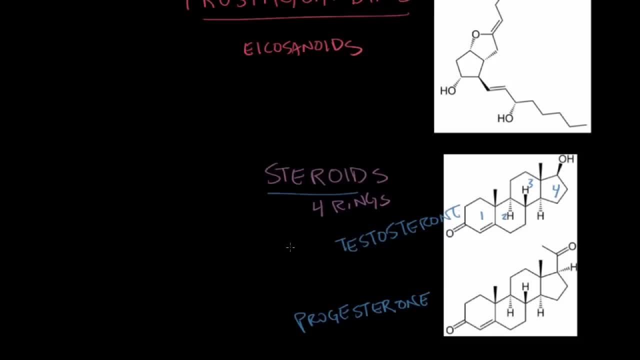 They signal things like puberty, for example. and then you have some other steroids like the corticosteroids- cortisone and aldosterone. But if you want to hear, I guess, a lot about steroids, you should definitely check out. 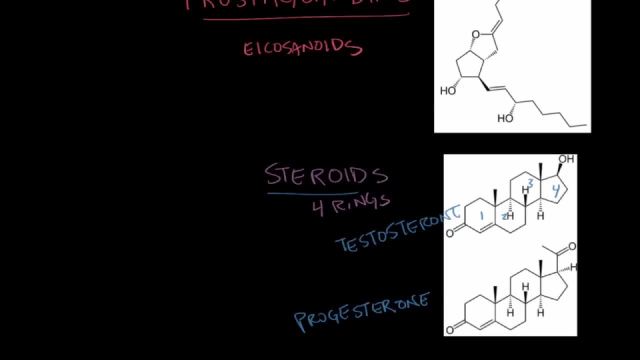 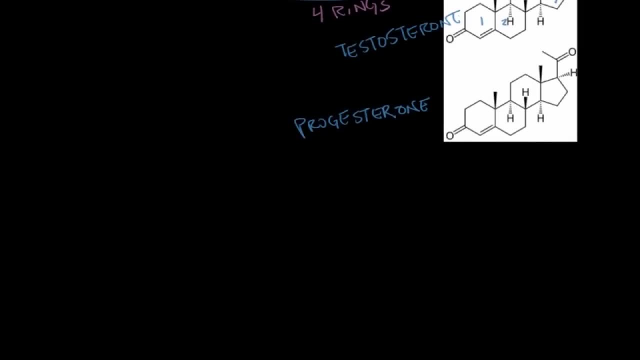 that other playlist of videos. But the last non-hydrolyzable kind of signaling lipid that I want to talk about are actually vitamins, so fat-soluble vitamins, And I suppose I misspoke a few minutes ago when I said that non-hydrolyzable lipids all. 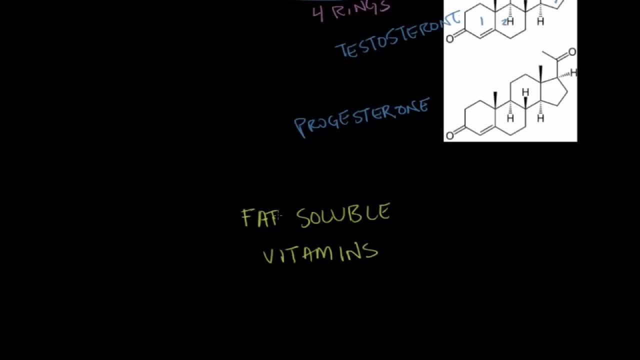 have this signaling function because fat-soluble vitamins really function more as coagulants, right Co-factors, so co-factors co-factors, which means that they help some enzyme in our body perform a function. Our cells don't make these compounds, so we have to ingest them to help these enzymes. 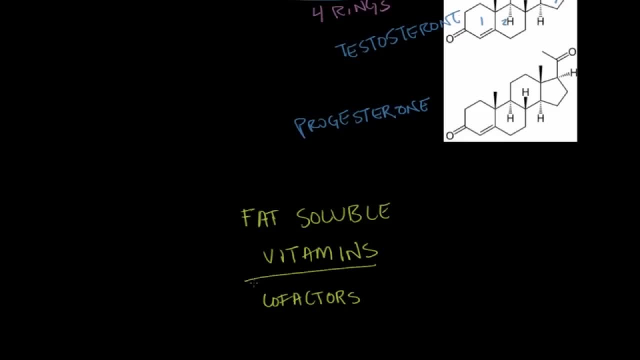 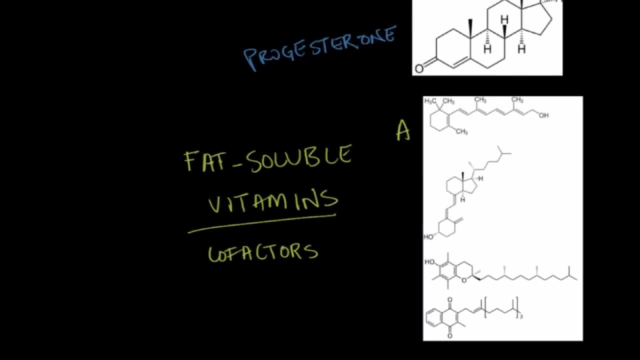 perform their function And there are four fat-soluble vitamins and we have A, D, E and K, And I think I've got a picture here that I can pull in for us. This one right here is A, And vitamin A is also called retinol and it's needed for light sensitivity in our vision. 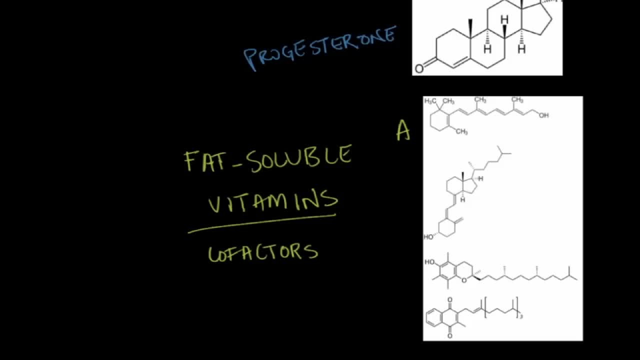 as well as kind of healthy mucous membranes. It has a couple different functions in our body. We have vitamin A. We also have vitamin D. Vitamin D helps regulate phosphorus and calcium metabolism, so deficiencies can cause a number of different bone diseases like rickets and 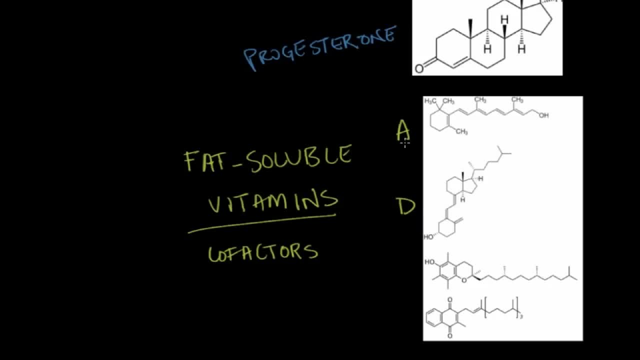 osteoporosis, And so we've got A, D, We've got E, We've got vitamin E right here. Vitamin E is an antioxidant that helps protect our neurological function- And then vitamin K. at the bottom we've got A D, E, and vitamin K regulates the synthesis.